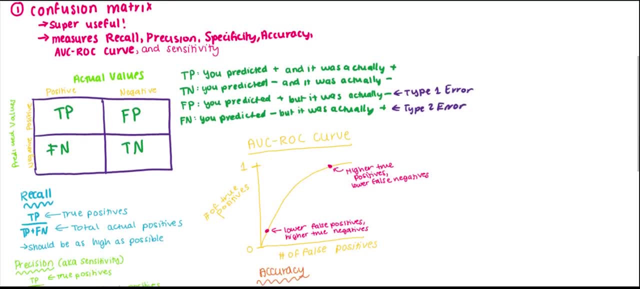 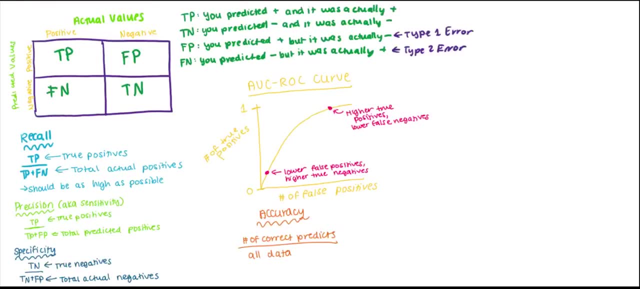 it was negative and it was actually negative. So these values can help you calculate some more performance metrics like recall, precision and so on. So let's look at how you can calculate those. You can calculate recall by taking the rate of true positives over the rate of true. 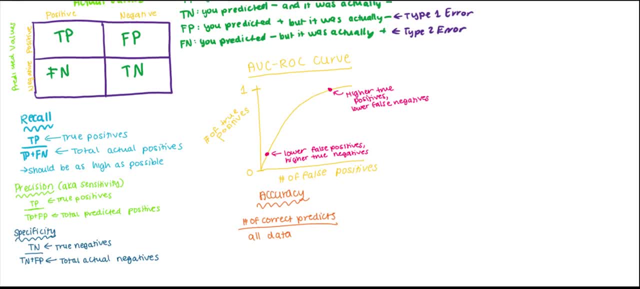 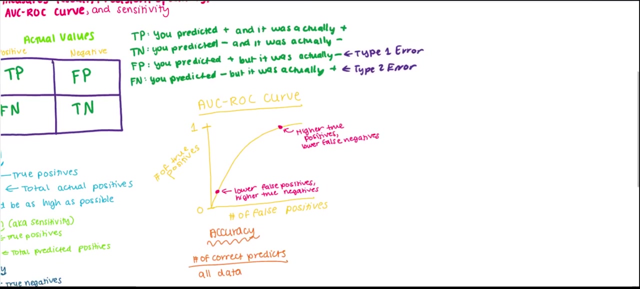 positives plus false negatives. You can calculate precision, which is also known as sensitivity, by calculating true positives over true positives plus false positives. You can calculate specificity by taking true negatives over true negatives plus false positives, And you can calculate accuracy by taking the total number of correct predictions over all the data. You can also look at the. 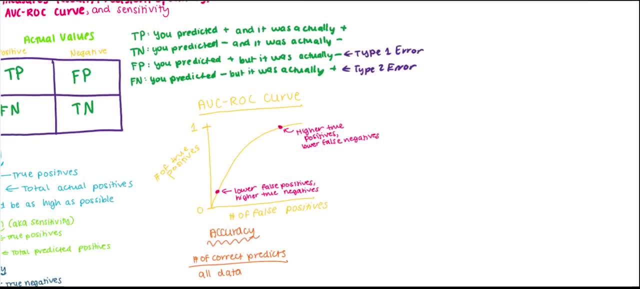 AUC-ROC curve, which is created using the number of false positives as the x-axis values and the number of true positives as the y-axis values, And they all range between 0 and 1.. So you can also use the AUC-ROC curve to interpret your data as well, And this is created using the help of a confusion. 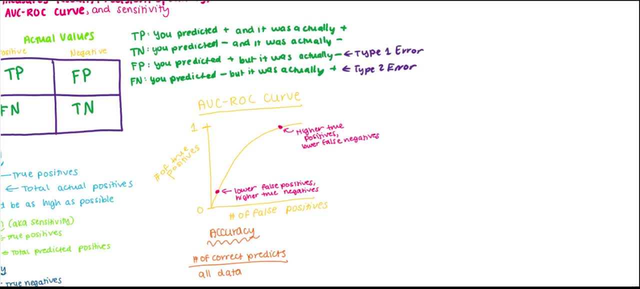 matrix, because you can see that the x-axis represents the number of false positives and the y-axis represents the number of true positives. So you can look at the values along the curve and interpret the data. For example, the lower the value is on the x-axis, like the bottom value over. 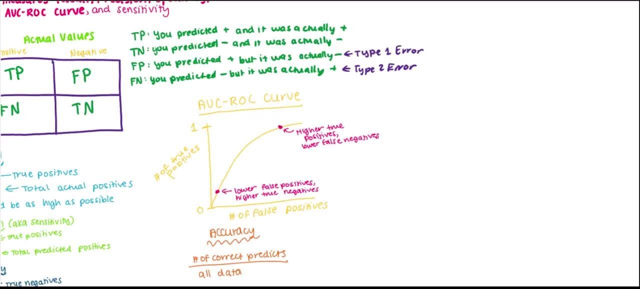 there that means lower false positives and higher true negatives. And if you look at values that are higher on the y-axis, that means higher true positives and lower false negatives. So if we go back to the example that I gave at the beginning of the video, you would see that accuracy actually 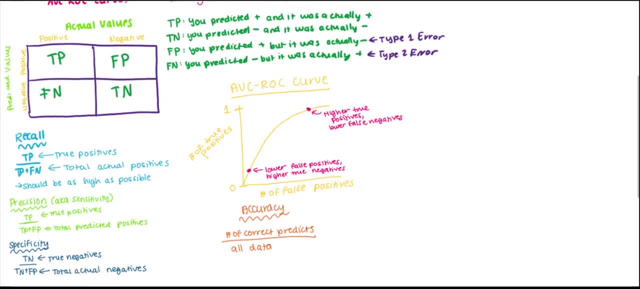 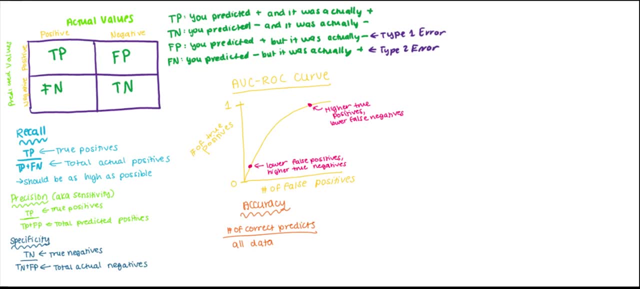 wouldn't be a very good measure of the model's performance, In my opinion. I think precision would be a much better measure of the model's performance. But you can also look at the value. you can also think to yourself what you think would be a better measure of the model's performance. 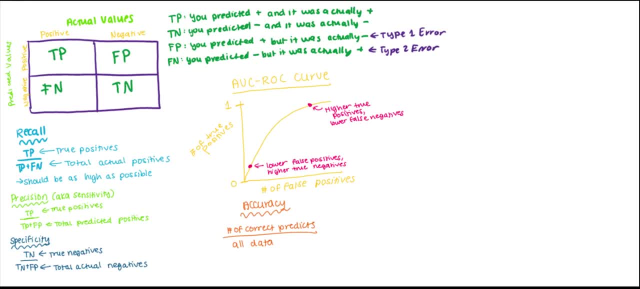 than accuracy, And you have to keep thinking when you're communicating your data to other people so you can accurately show what the precision of your machine learning model is. As always, if you have any questions, you can leave a comment below or email contact at AIinspiredorg. Thank you so much.